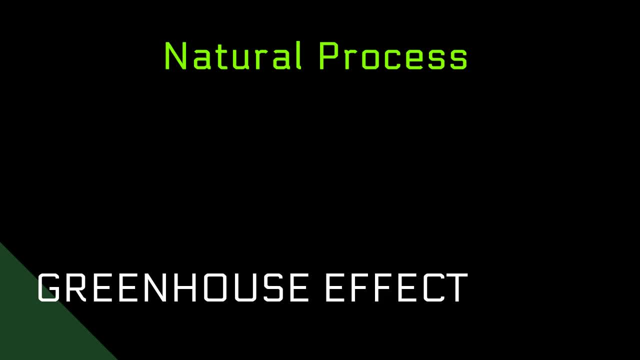 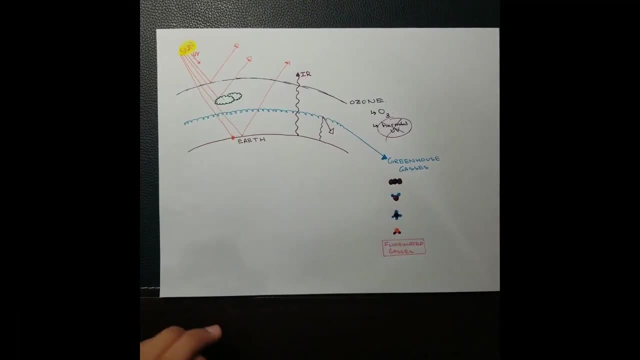 on Earth. If there were no greenhouse gases, Earth's average temperature would be around zero degrees Fahrenheit, or negative 18 degrees Celsius. However, greenhouse gas levels have been rapidly increasing recently, leading to global warming. Greenhouse gases consist of carbon dioxide, or CO2, water vapor, or H2O- carbon dioxide. 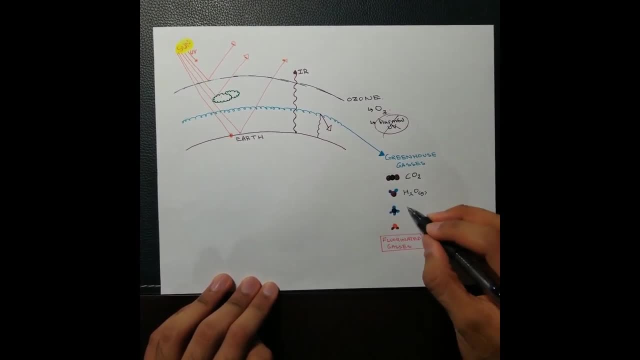 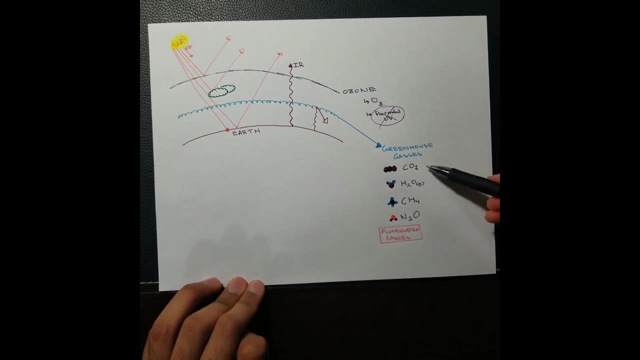 or CO2, and water vapor or CO2.. Methane or CH4, nitrous oxides or N2O and fluorinated gases. CO2 is mainly emitted from burning fuels like natural gas, coal and wood. It can also 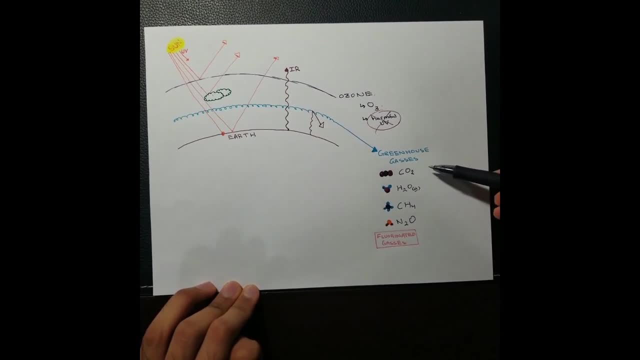 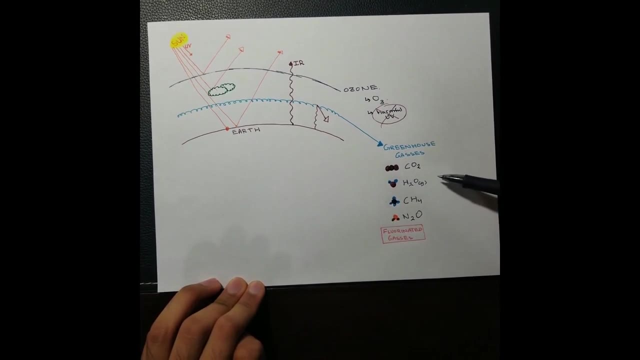 be emitted from respiration and the manufacturing of certain goods. CO2 is naturally sequestered by photosynthesis, but CO2 levels have been increasing due to increased fossil fuel usage. Water vapor is created from the evaporation of water. As the globe heats up, more water. 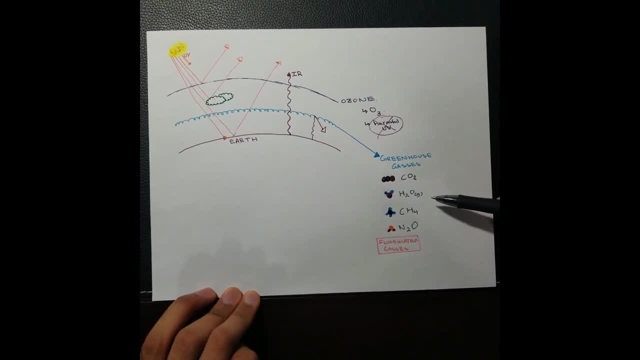 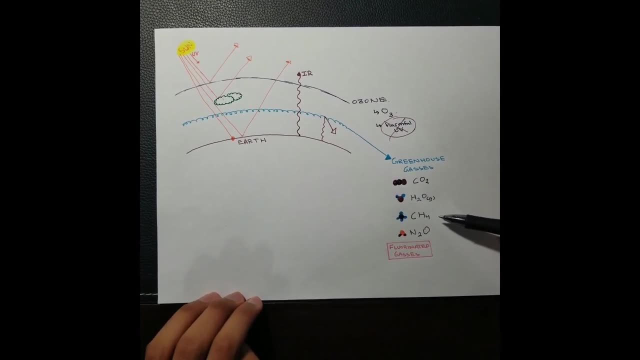 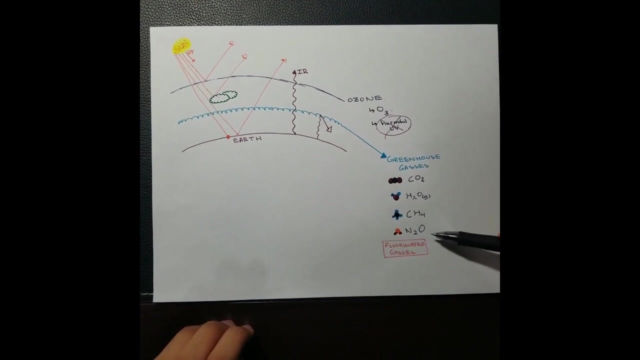 is evaporated. Methane is emitted from livestock, agriculture, waste management, industrial processes and leaked natural gas. It has a shorter lifespan than CO2, but is 25 times worse. Nitrous oxide gets emitted due to agricultural and industrial processes. fuel combustion. 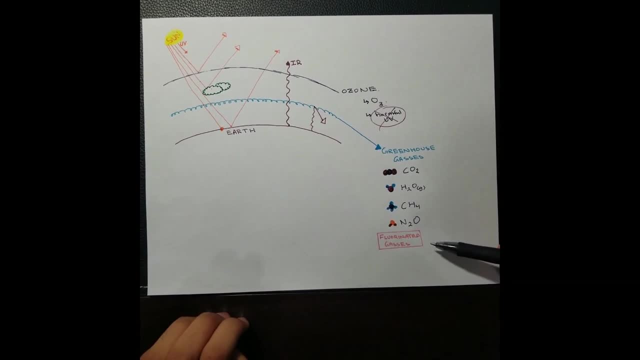 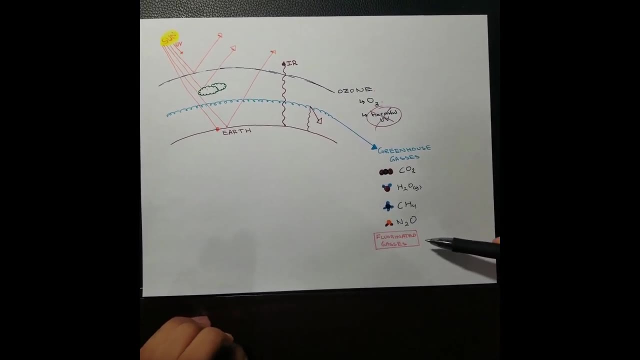 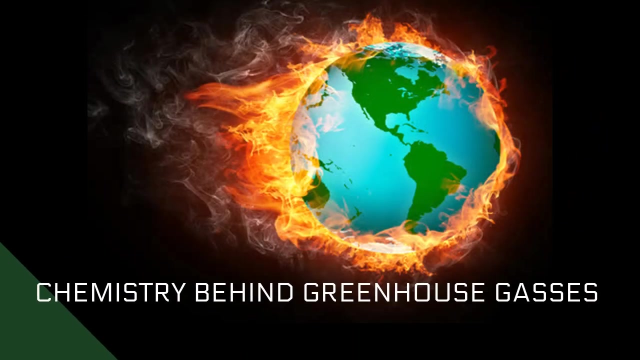 and that is part of the natural nitrogen cycle. Fluorinated gases come only from synthetic processes such as semiconductor manufacturing and insulation. They are the most harmful type of greenhouse gas and function by depleting the ozone layer. Infrared radiation causes greenhouse gases to vibrate more and collisions between molecules 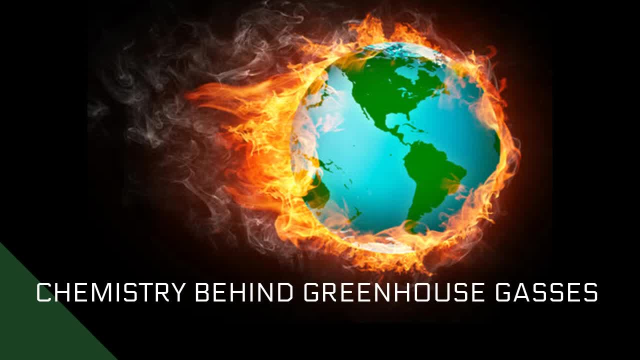 that transfer vibrational energy increase, thus increasing the average thermal energy. Only molecules that have three or more atoms can absorb the infrared radiation. Oxygen gas, nitrogen gas and argon together make up 99.9% of the total carbon dioxide in the.